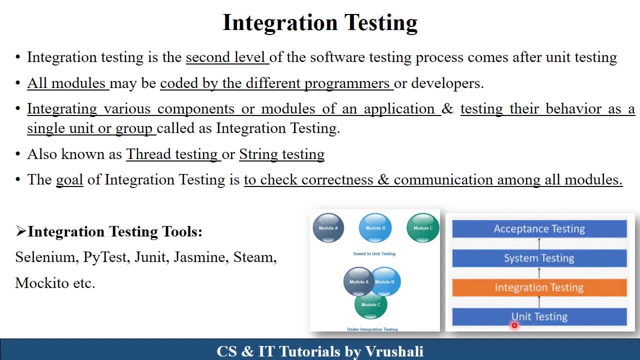 testing is a first level of testing. Here tester test each and every modules, components, functions, methods mentioned in your program, individually or separately. After unit testing there is integration testing. The name suggests that integration Means here. tester combine or integrated all the modules in your program. 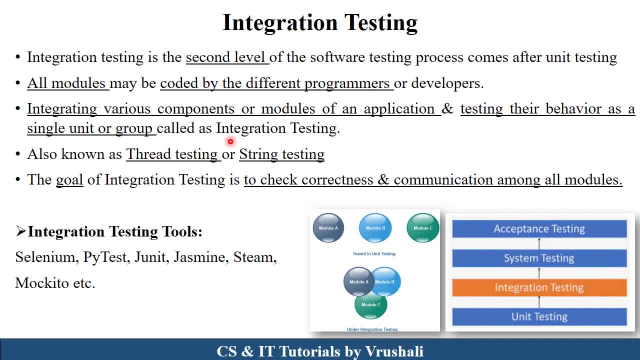 And after that they perform testing on that. See, in particular project there are different types of modules are present. Now this: all types of modules are developed by different programmers or the developers. Now in integration testing tester integrate all these components and modules into the single group. Basically they perform testing on complete project or 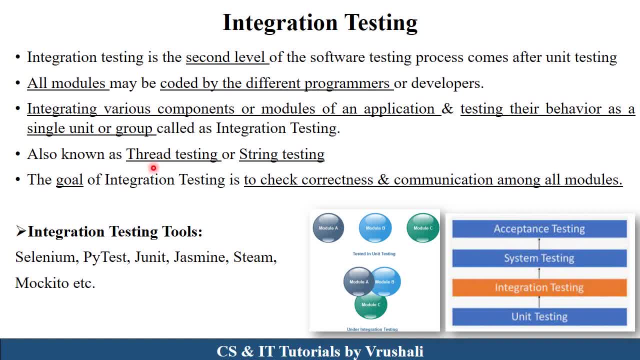 complete program. That's why, which is also called as threat testing or threat testing. The main goal of integration testing is to check correctness, accuracy, quality and communication between all the other modules. There are different integration tools are available in market, like selenium, pytest, JUnit, Jasmine, Now tester. use those tools. 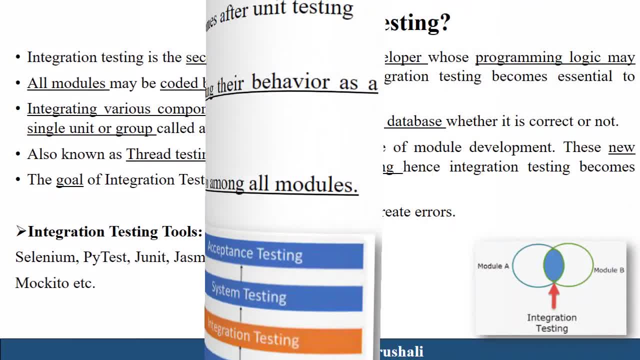 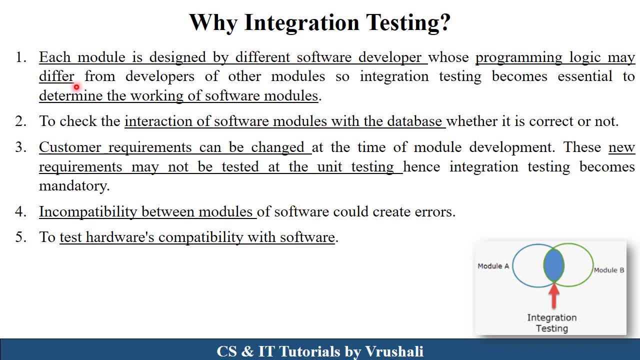 for generating different types of test cases. The next topic is: why integration testing? As we discussed earlier In project, there are different types of modules. These modules are developed by design by different types of software developers. Their programming logic may be also different, right, So integration. 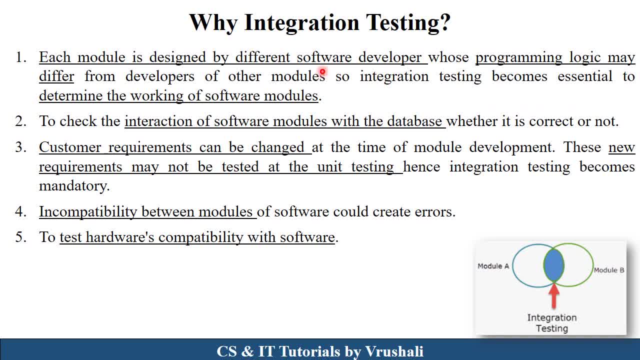 testing, combine or integrate all these modules and after that performing operation on that Integration testing, also check that interaction of different software modules with the database- In your project there are different modules- is interact with the database. They perform insert, Delete this kind of operation on the database. So here integration testing, test their interaction. 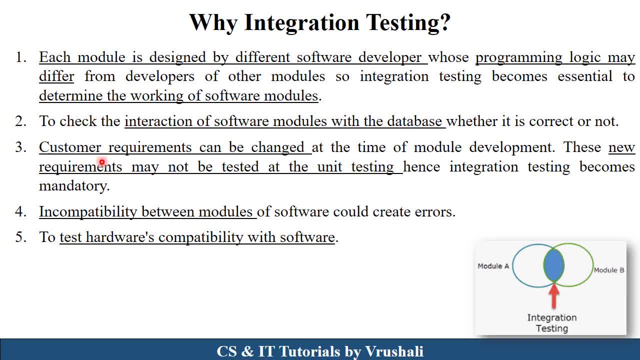 and accuracy of the result. Sometimes in your project customer requirements are continuously change. Now this- all the new requirements- may not be tested at the unit testing, So at that time this new requirements are tested in integration testing process. In your project there are different types of models, For example in college management system project there. 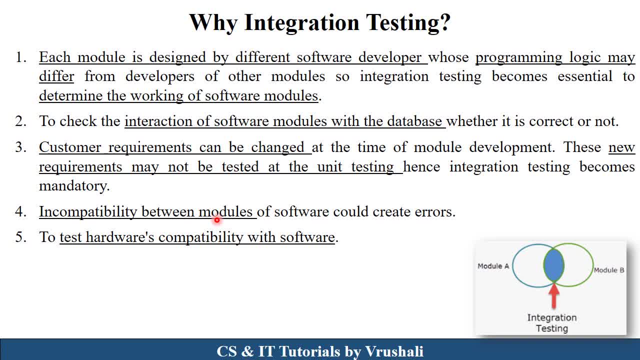 are teacher module, HOD module and students module. So this- all three modules are interrelated with each other. They share information with each other. So integration testing test their compatibility and data flow between all this modules. Integration testing also test the compatibility of hardware and software used in your project. That's why integration testing 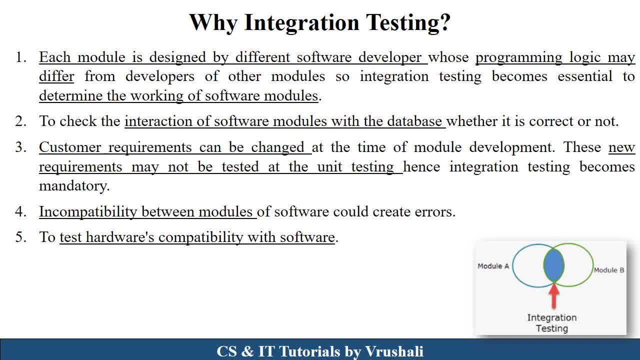 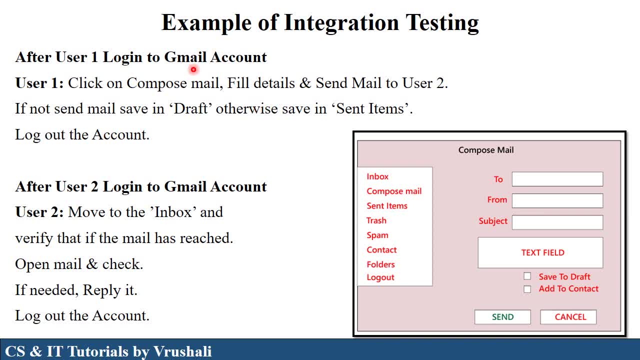 is one of the most important testing in software testing process. See here in this particular example. this is just a basic example of Gmail account. I think you all are familiar with the Gmail right. Suppose user 1 log in to particular Gmail account and they want to send mail to the user 2, right. 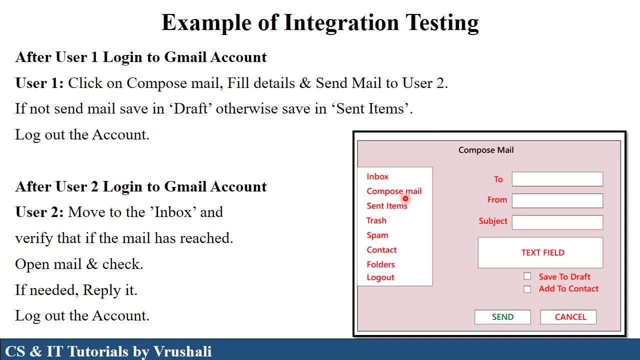 For that purpose. first they click on compose mail option, After that they fill all the required details like to from subject, and after that they send mail to the user 2.. Now this sending mail is saved into the send items folder. 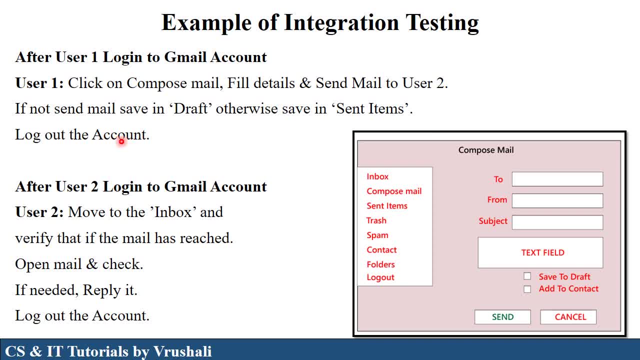 After that, user 1 log out particular account. Now next thing is user 2.. So user 2 log in their Gmail account and move to particular inbox folder And they verify that a particular mail has received or not. right After opening a mail, they check a particular mail and, if needed, they give a proper reply to user 1.. 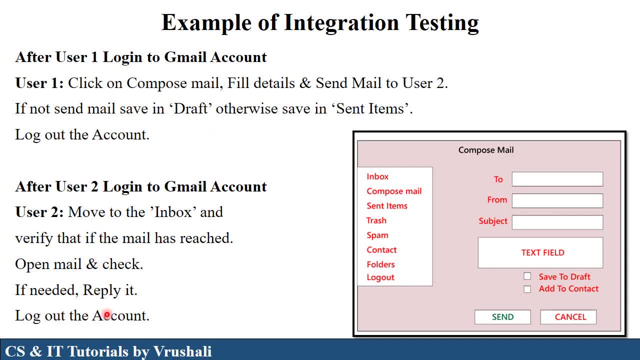 And at the end they log out. So in integration testing tester check this complete process are properly occur or not. In unit testing they test each and every components or functionality are properly work or not. But in integration testing they test that this complete process of sending mail is properly work or not. 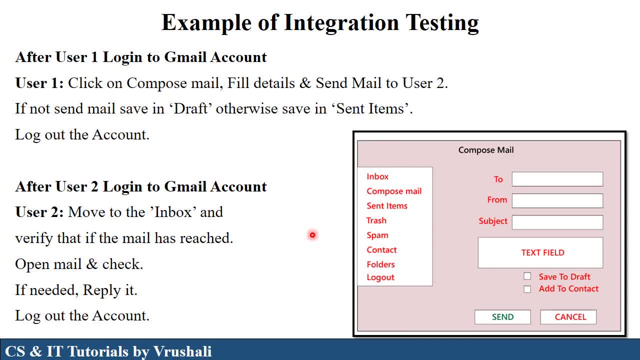 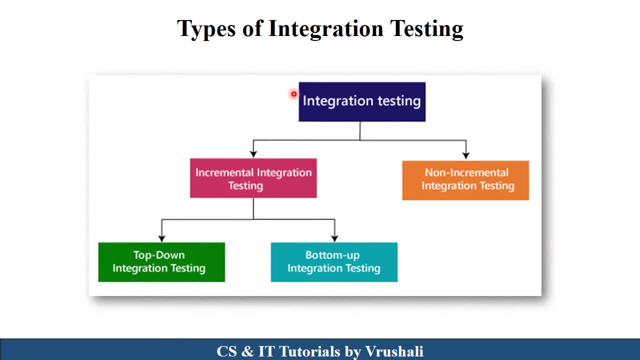 So this is called as integration testing. They integrate all these modules and check their data flow and correctness of the result. They integrate all these modules and check their data flow and correctness of the result. Now the next topic is types of integration testing. Integration testing mainly divided into the two types like incremental and non-incremental integration testing. 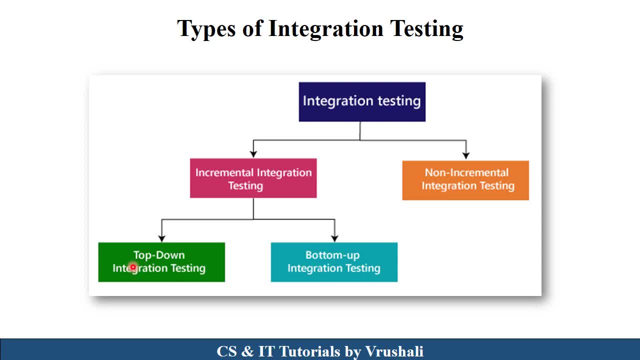 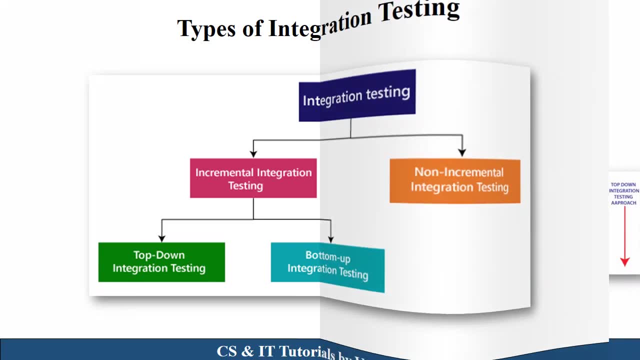 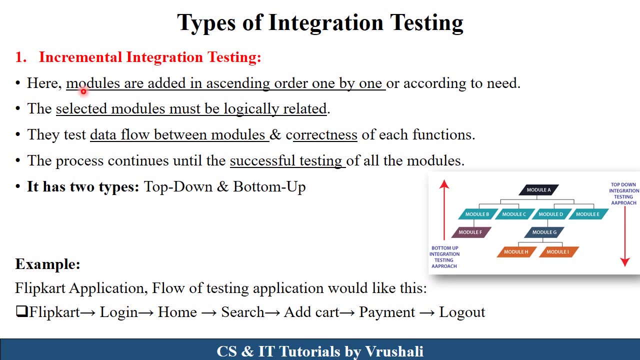 This incremental testing again divided into the two types like top-down and bottom-up integration testing. Now let's discuss this- all types of testing- in detail. The first type of testing is incremental integration testing. Here, Tester, add all the modules in your project in ascending order, one by one for testing purpose. 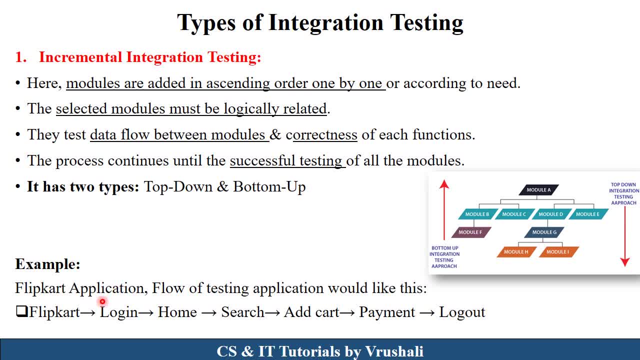 Just take a example. See here: suppose in flipkart application user first open a flipkart for that purpose they use login process. After that the first page is home page. Now they search a particular product. If user like a particular product, they add a particular product into the add cart option. 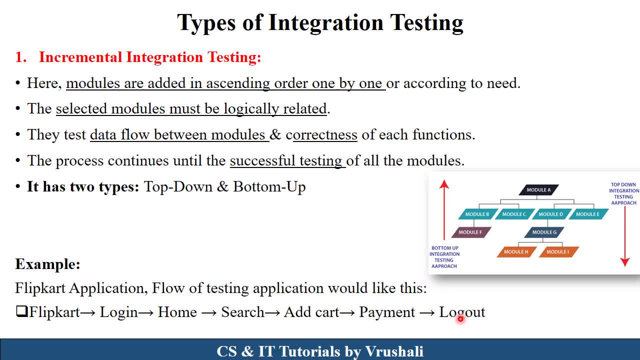 Right After that they perform page search, They check the payment and logout the application. So this is a particular process. So in incremental integration testing here, tester check that this particular process from top to bottom or from start to end, is properly occur or not. 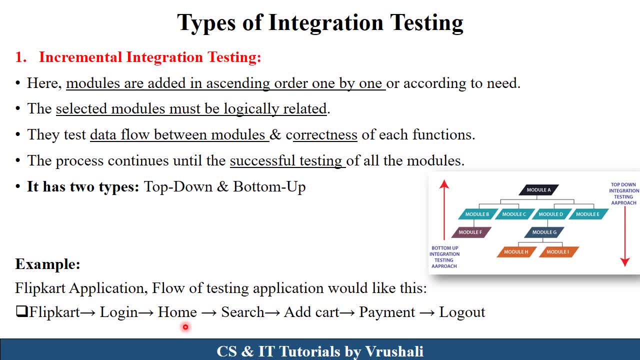 So this is called as incremental integration testing. Here tester check data flow between all these modules and functionality and check their correctness of the result. This process continue until successful testing of all modules. So this is called as incremental integration testing. Here tester check data flow between all these modules and functionality and check their correctness of the result. 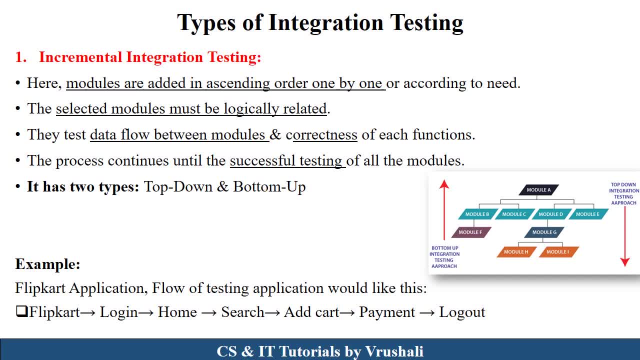 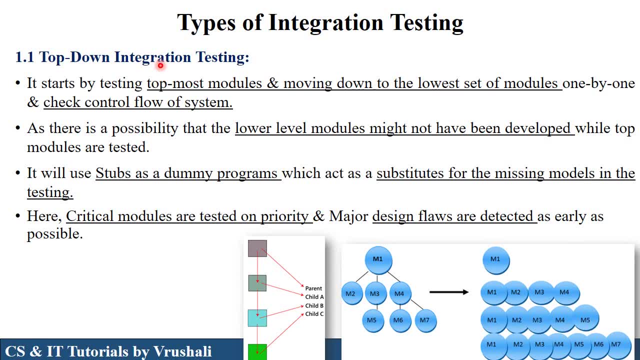 This incremental integration testing divided into two types, like top down and bottom-up integration testing. Now let's discuss these types in detail. The first type of testing is top down integration testing. In your particular program you have to mention first parent class. after that you have to mention that child class, right like child a, child B and child C. 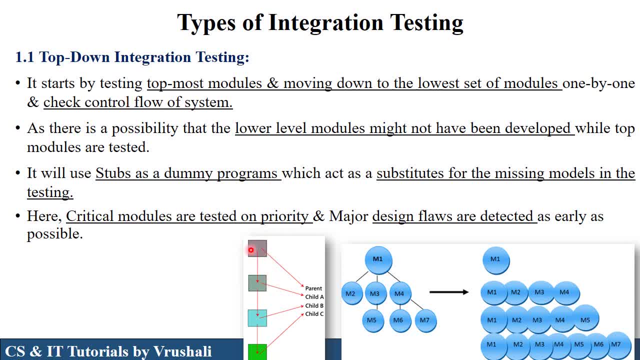 So in top down integration testing, down integration testing, here tester test first parent class, after that they test parent class and child a class, after that they test parent, a, parent class, child a and child b class, and after that they test parent, child a, child b and child c class. so this is called. 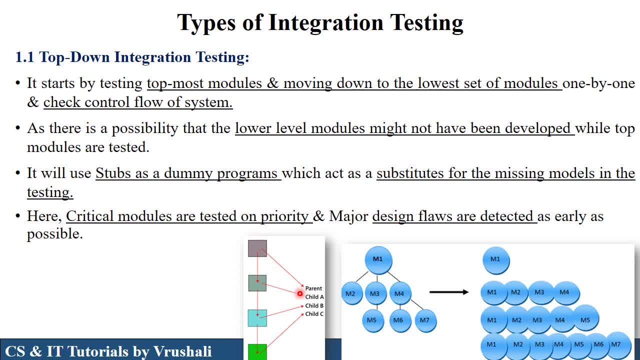 as top down integration testing. they perform or analyze the flow of data or flow of output of particular program. see here in this particular image. this is a hierarchical structure of top down integration testing. first there is a m1 module, so tester test. first m1 module, that is topmost module under m1. there is a m2, m3 and m4 module, so tester test- m1, m2, m3. 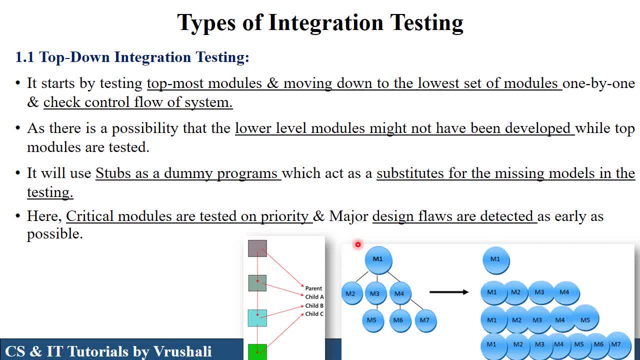 m4 module in the separately right. so they integrate each and time different parent to child class. so this is called as top down integration testing. sometimes what happen this? m1 and m3 modules have develop but m5 module is remain to develop right. so at that time they use a dummy module here for testing purpose. and this dummy module. 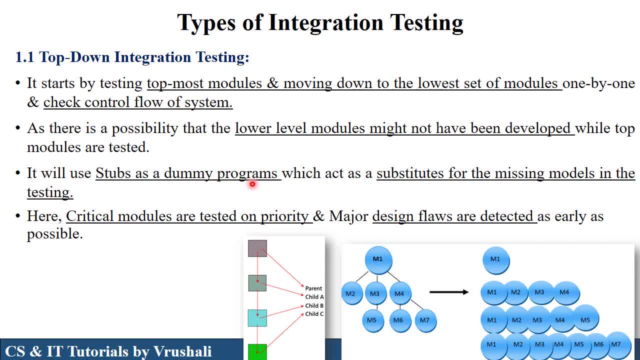 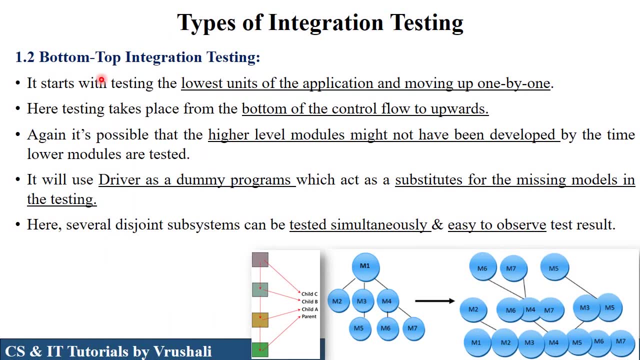 is called as STERP. STERP act as a dummy program and which act as a substitute for the missing model for testing purpose. right, so they check their data flow between all this module. this is called as top down integration testing. now the next type of testing is bottom to top integration testing. so this is just a 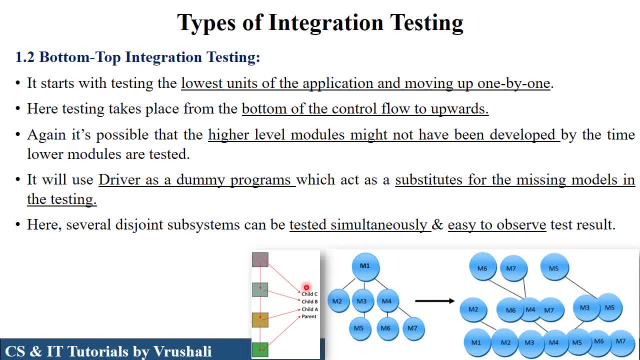 opposite of top down integration testing. see here in this particular image: here tester test first child c class, after that they test child c and child b class. they are working their flow. after that they test child c, b and child a class, and after that they test child c, b and their parent class. so basically they test the complete flow between child. 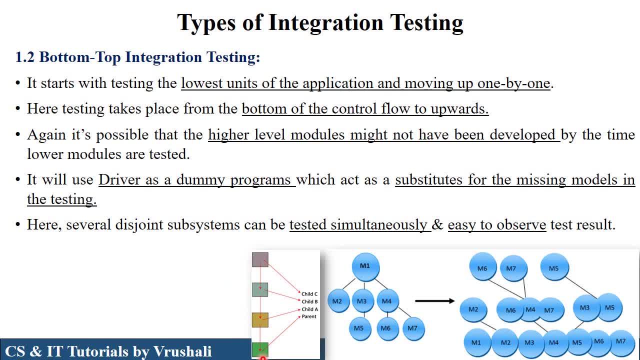 to parent class. so this is called as bottom to top integration testing. see here in this particular hierarchical structure here in integration testing tester test first m6, m7 and m5 module. after that they test their combine module or integrated module. in this way sometimes what happen in bottom to top integration testing: m5, m3, these two models are already develop. 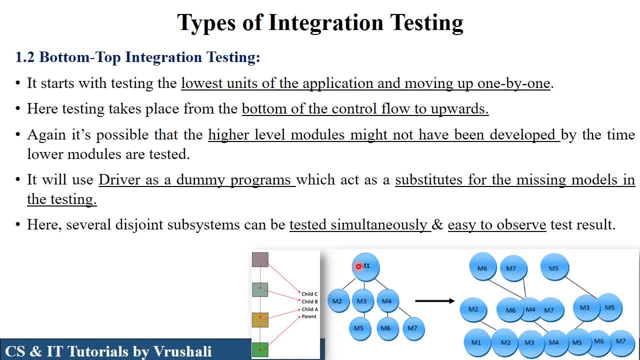 but m1 module is still for remain in this particular hierarchical structure, here in this particular integration testing. you can do the follow up test here: m6, m2 and m6 and m5 module in the remaining right. so for this remaining module they use a driver as a dummy program. okay, 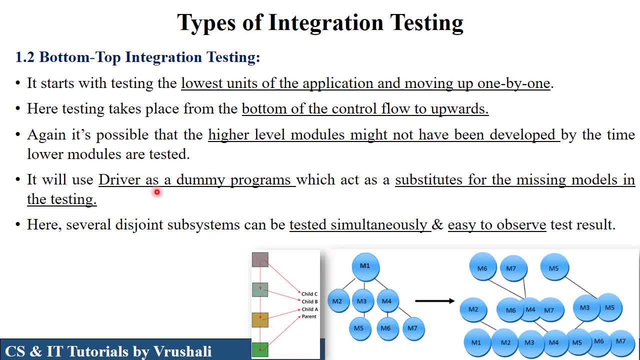 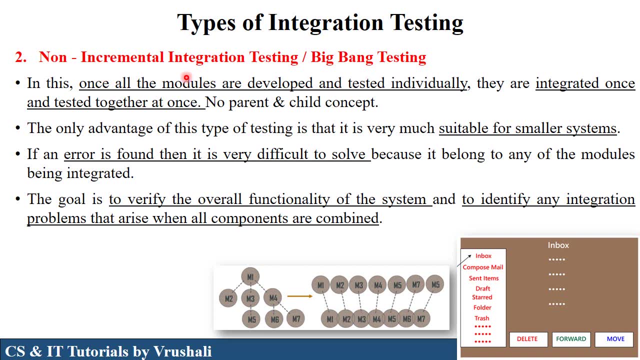 so they test for testing purpose. they just use this dummy model or dummy program and they test that each and every modules are properly work or not, and they test their accuracy result of each and every modules. now the next type of testing is non incremental integration testing, which is also called as big bang testing. see in previous types of testing we discuss. 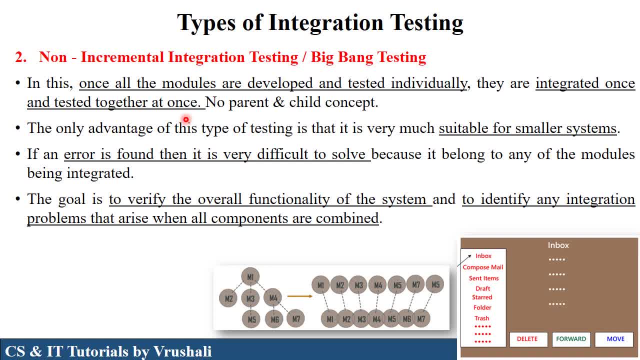 they test each and every modules and integration of that modules, right. so once all the modules are developed and tested individually, after that non incremental integration testing is work. so here, non incremental testing, work on complete integrated module or complete project when your project is completely developed. so they check a final result and then they 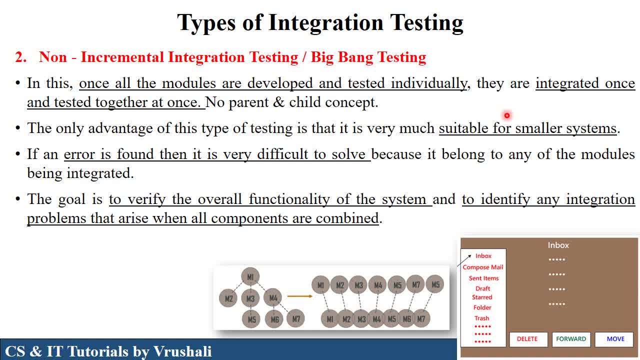 check the final result and final output of your project. so this non incremental integration testing is suitable for this smaller system, suppose at that time, if errors are found, so it is very difficult to solve because it is very difficult to identify in which modules errors have occurred. right see here in this particular image. here is a m1, m2, m3, m4 after. 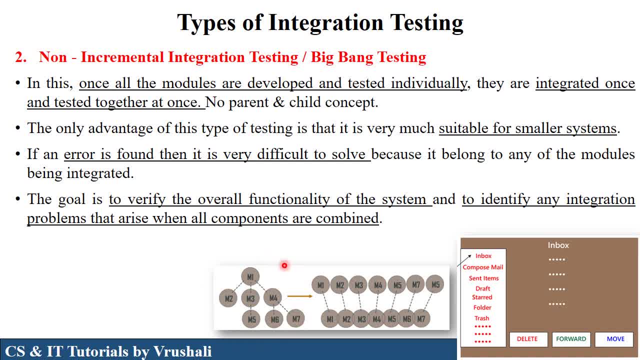 that m5, m6, m7, this modules are completely developed. so non incremental integration testing. these all modules test accurately or separately. right see here in this particular example. suppose in particular gmail account there is a inbox option, is there so inbox, having no any parent class or child class, right after that, compose mail, sent atoms. so after developing, 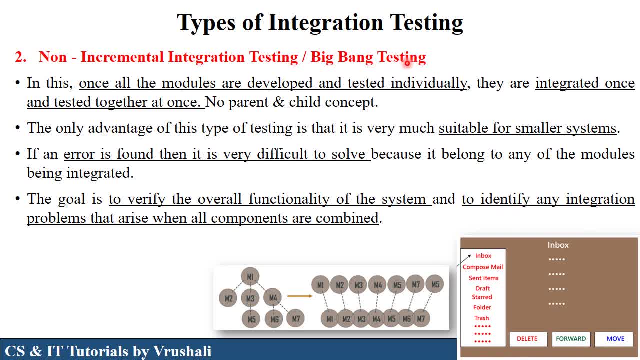 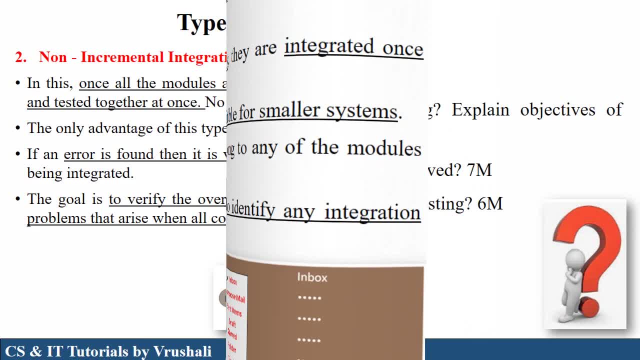 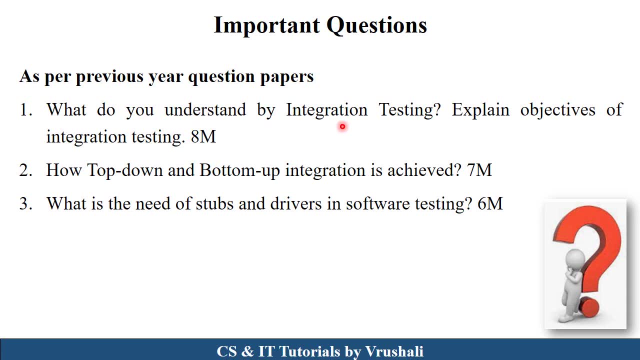 a complete gmail application here, big bang testing its work. they test complete particular product or the project at a same time. now, as per your previous year question papers, these questions are important like: what do you understand by integration testing? explain objectives of integration testing for 8 marks. how top down and bottom of integration testing is achieved for 7 marks. 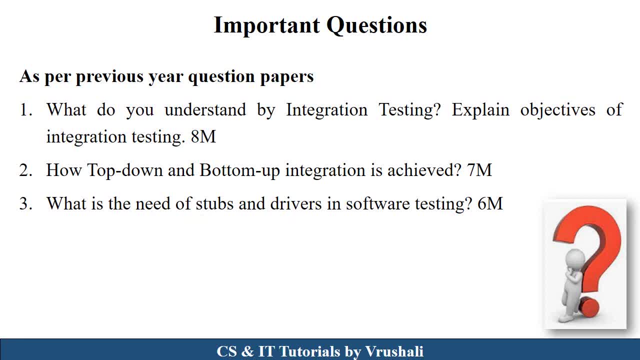 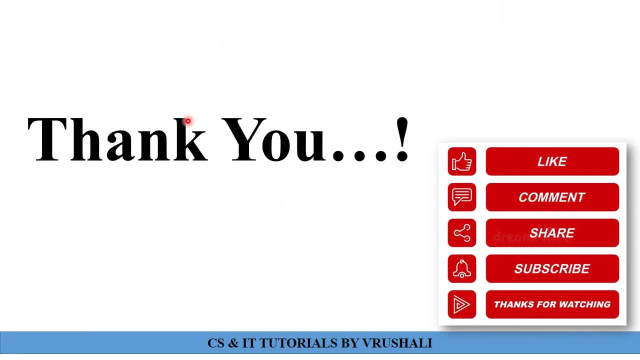 and what is the need of stops and drivers in software testing for 6 marks. so you have to prepare this topics completely. so this is all about integration testing. thank you, keep learning.